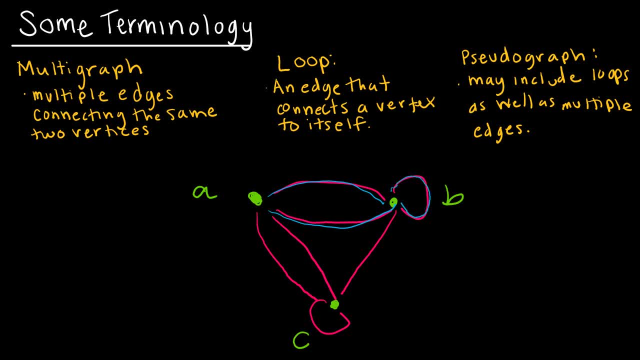 however, again we talked about that a little bit. a loop connects a vertex to itself. A multigraph actually would not contain any of those loops, but a pseudograph is what I have pictured here, which contains both multiple edges and loops, So it could include one or both. We've already spoken a little bit about digraphs, or 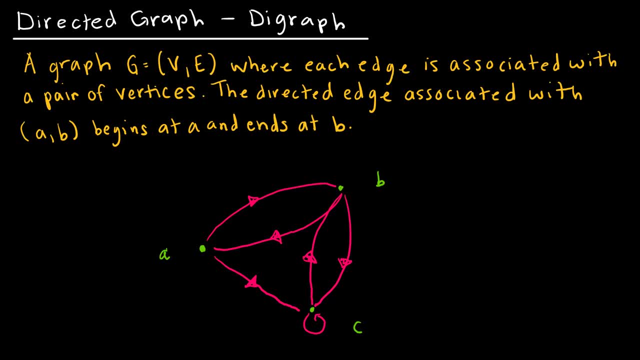 directed graphs- and this is just a graph- where each edge is associated with a pair of vertices. So the directed edge associated with A- B begins at A and ends in B, etc. So if we were to list the vertices included in this directed graph, we would have A- B, because A goes to B. So 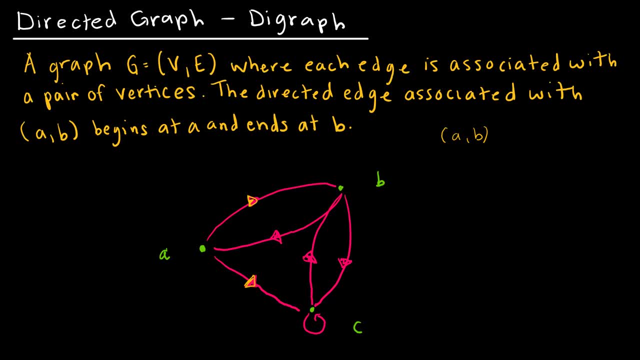 I've used this one and I would also have A, C, because A goes to C And then, looking at B, I've got one from B to A, So BA would be two points here: B to C And then from C. I have C to B. 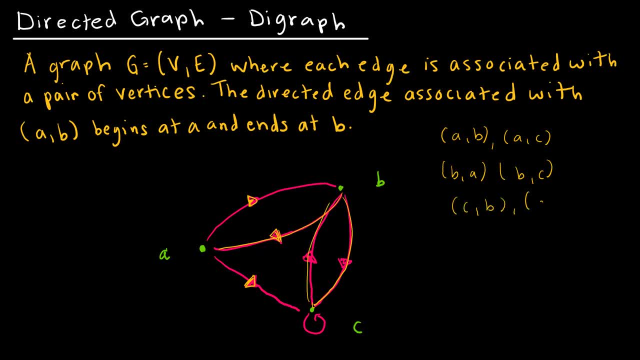 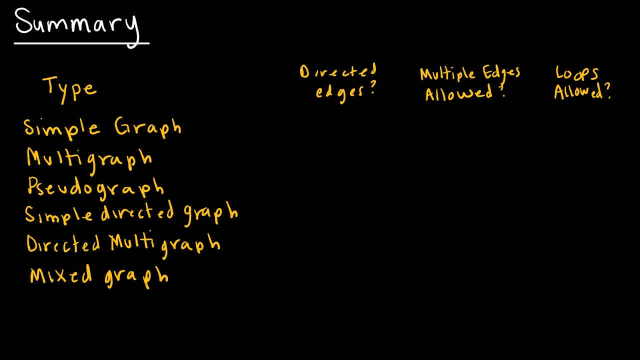 And I also have C unto itself, So these would be the ordered pairs that would be associated with this particular directed graph. So hopefully I can help you sort out some of this terminology to make sure that we're on the right track here. So I've got several types of graphs listed: Simple graph. 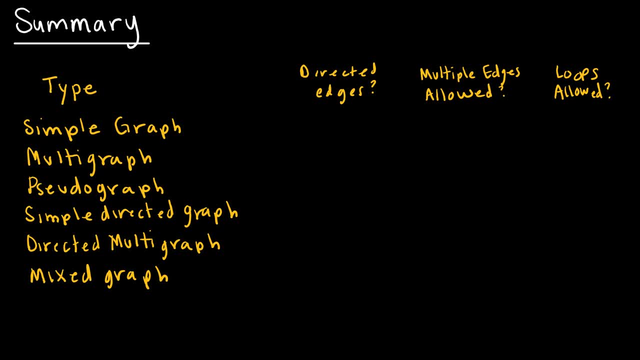 multigraph, pseudograph, simple directed graph, which we didn't talk about, explicitly directed multigraph and a mixed graph, And we're going to talk about what kind of properties these graphs will have. So we know a simple graph does not have directed edges, It's just regular edges. so there's no arrows. 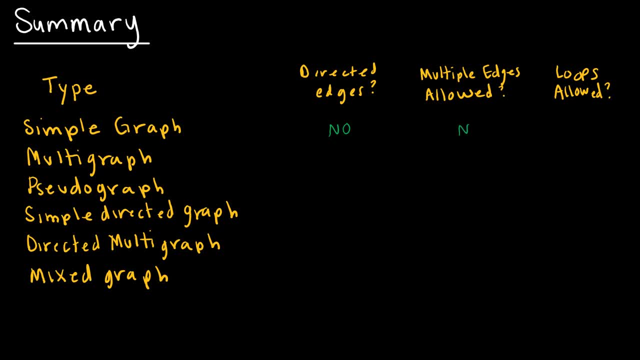 Can I have multiple edges? Can I have multiple edges? Can I have multiple edges on a simple graph? No, I cannot, because otherwise it would not be simple. And can I have loops? No, because the definition of a simple graph is essentially no. 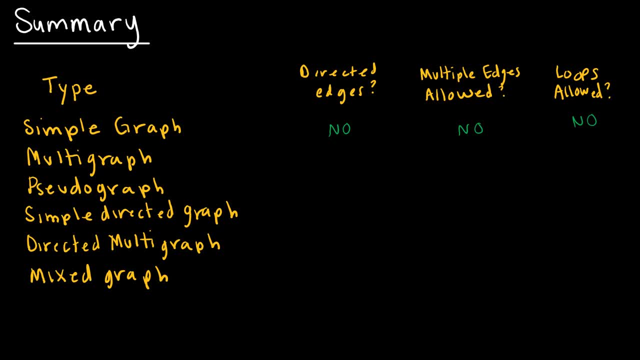 multiple edges and no loops. Now we talked about a multigraph. A multigraph said you can have multiple edges connecting the same two vertices. So again, still not directed. but yes, multiple edges are allowed, but I still cannot have loops. A pseudograph is still not directed, but it can have.